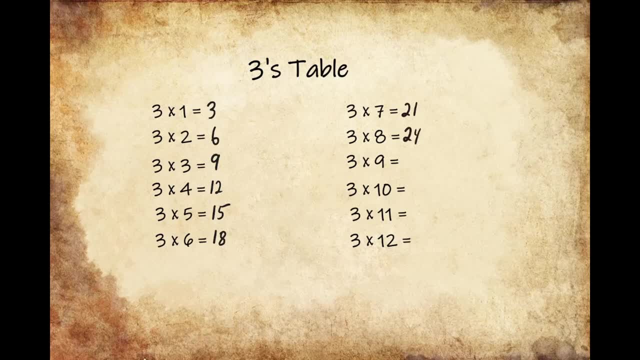 21,. 3 times 8 gives us 24,. 3 times 9 gives us 27,. 3 times 10 gives us 30,. 3 times 11 gives us 33, and 3 times 12 gives us 36.. Now, looking at the fours table, 4 times 1 gives us 4,. 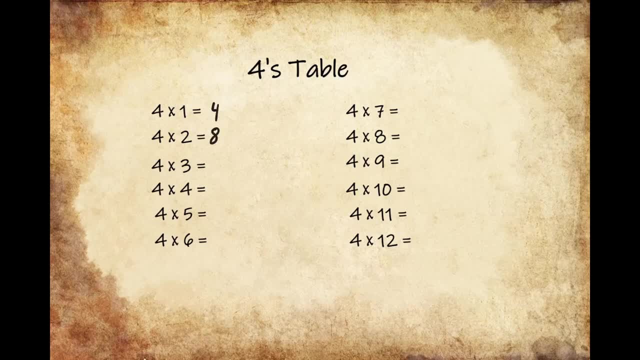 4 times 2 gives us 8,. 4 times 3 gives us 12,. 4 times 4 gives us 16,. 4 times 5 gives us 20,. 4 times 6 gives us 24,. 4 times 7 gives us 28,. 4 times 8 gives us 32,. 4 times 9 gives us. 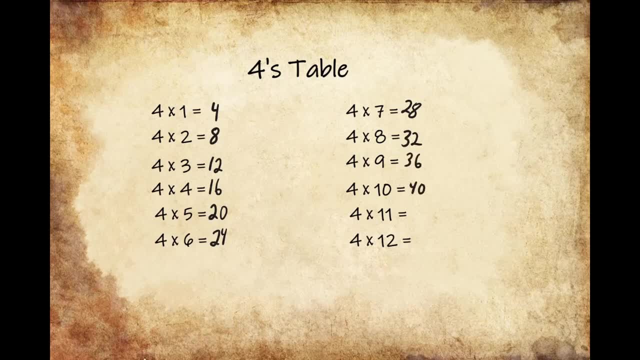 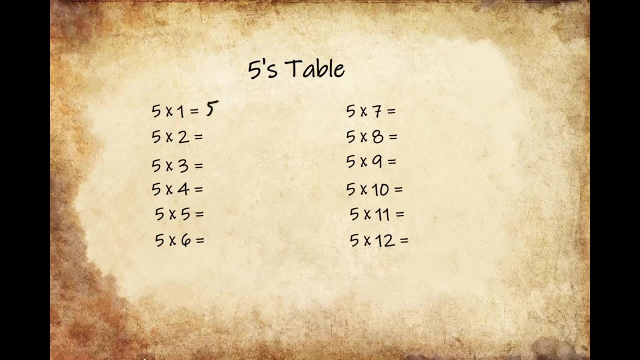 36,. 4 times 10 gives us 40,, 4 times 11 gives us 44, and 4 times 12 gives us 48.. Now we're looking at the five times table: 5 times 1 gives us 5,. 5 times 2 gives us 10,. 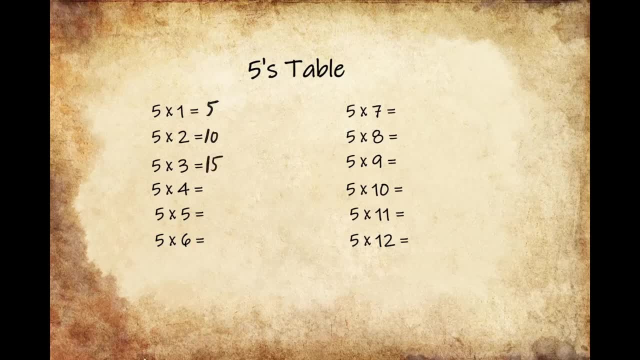 5 times 3 gives us 15,. 5 times 4 gives us 20,. 5 times 5 gives us 25,. 5 times 6 gives us 30,. 5 times 7 gives us 35,. 5 times 8 gives us 40,. 5 times 9 gives us 45,. 5 times 10 gives us 50,. 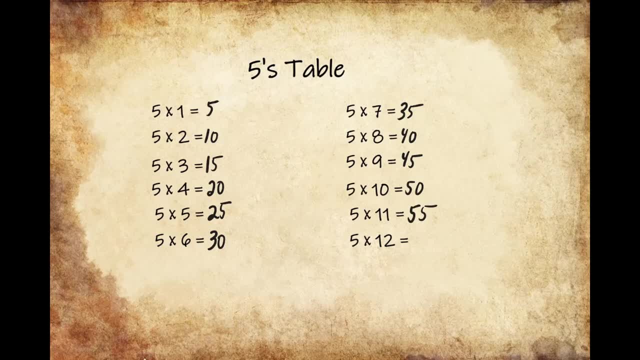 5 times 11 gives us 55, and 5 times 12 gives us 60.. Looking at the six times table, 6 times 1 gives us 6,. 6 times 2 gives us 12,. 6 times 3 gives us 18,. 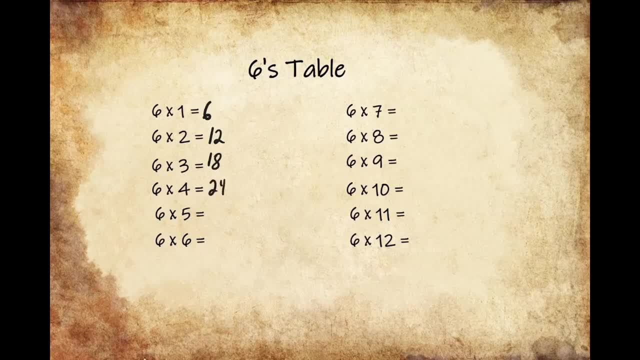 6 times 4 gives us 24,. 6 times 5 gives us 30,. 6 times 6 gives us 36,. 6 times 7 gives us 42,. 6 times 8 gives us 48,. 6 times 9 gives us 54,. 6 times 10 gives us 60,. 6 times 11 gives us 66,. 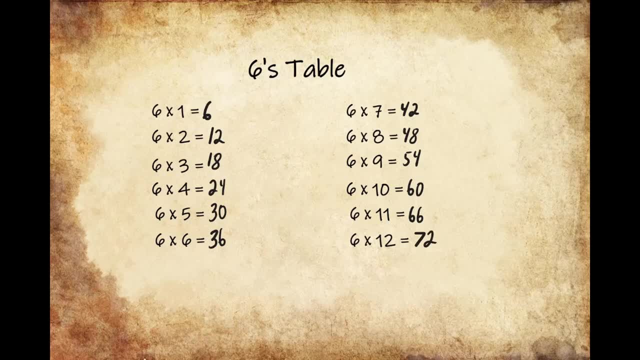 and 6 times 12 gives us 72.. Now for the sevens table. 7 times 1 gives us 7,. 7 times 2 gives us 14,. 7 times 3 gives us 21,. 7 times 4 gives us 28,. 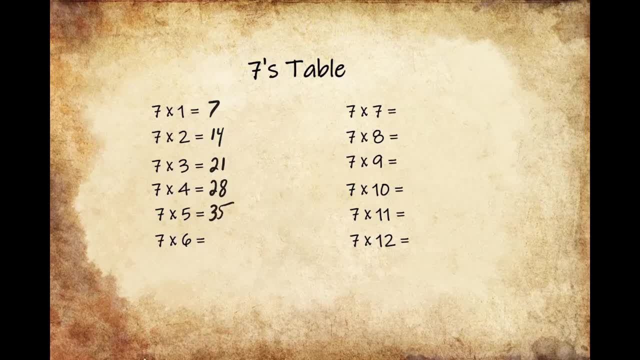 7 times 5 gives us 35,. 7 times 6 gives us 42,. 7 times 7 gives us 49,. 7 times 8 gives us 56,. 7 times 9 gives us 63,. 7 times 10 gives us 70,. 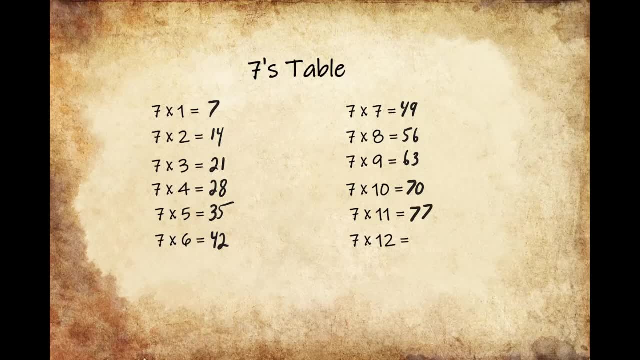 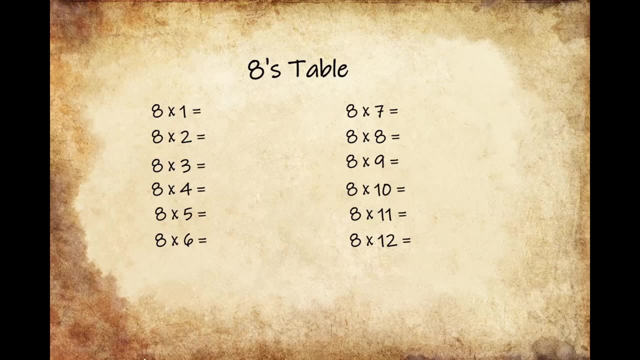 7 times 11 gives us 77, and 7 times 12 gives us 84.. Now, looking at the eights table: 8 times 1 gives us 8,. 8 times 2 gives us 16,. 8 times 3 gives us 24,. 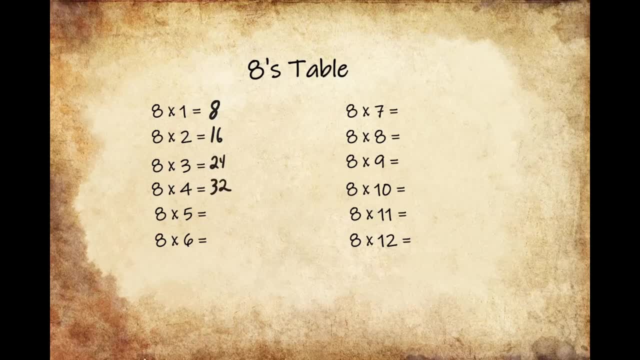 8 times 4 gives us 32,. 8 times 5 gives us 40,. 8 times 6 gives us 48,. 8 times 7 gives us 56,. 8 times 8 gives us 64,. 8 times 9 gives us 72,. 8 times 10 gives us 80,. 8 times 11 gives us 88,. 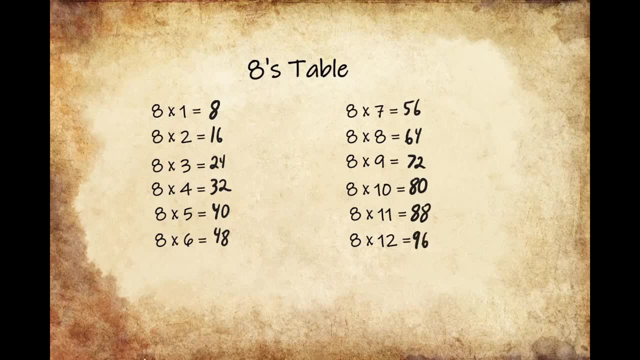 and 8 times 12 gives us 96.. Now for the nines table: 9 times 1 gives us 9,. 9 times 2 gives us 18,. 9 times 3 gives us 27,. 9 times 4 gives us 36,. 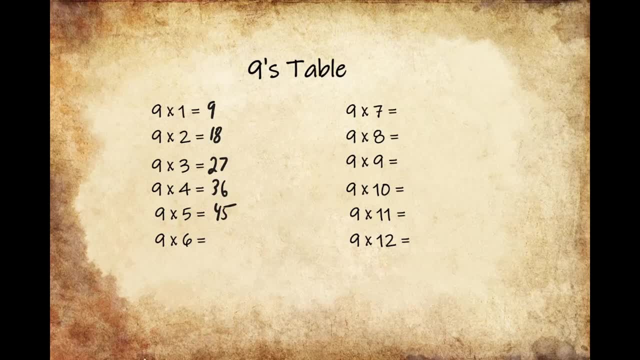 9 times 5 gives us 45,, 9 times 6 gives us 54,, 9 times 7 gives us 63,, 9 times 8 gives us 72,, 9 times 9 gives us 81,, 9 times 10 gives us 90,, 9 times 11 gives us 99, and 9 times 12 gives us 108. 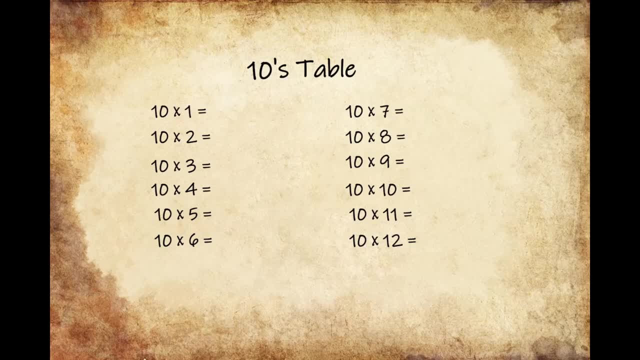 Now for the nines table, And now for the tens table. 10 times 1 gives us 10,. 10 times 2 gives us 20,. 10 times 3 gives us 30,. 10 times 4 gives us 40,. 10 times 5 gives us 50,. 10 times 6 gives us 60,. 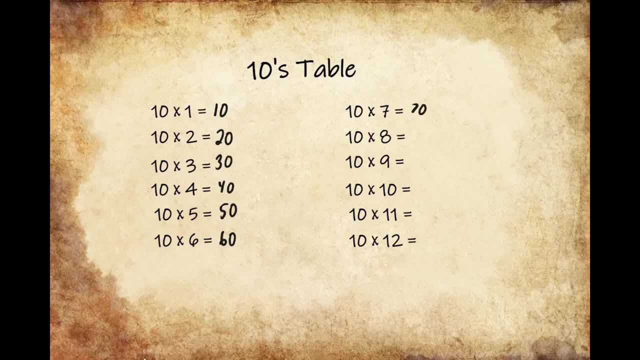 10 times 7 gives us 70,, 10 times 8 gives us 80,, 10 times 9 gives us 90,, 10 times 10 gives us 100,, 10: 11 gives us 110, and 10 times 12 gives us 120..